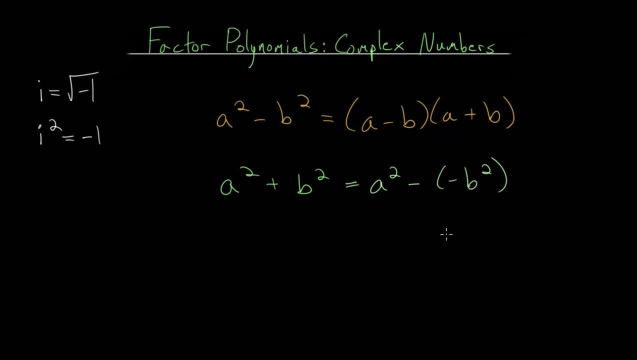 be able to rewrite this as a squared minus i squared times b squared. And so we go ahead and recognize that this is going to be divided by a squared plus b squared. On the tip of the that, right now we know that it's going to be a squared plus a squared plus a squared. 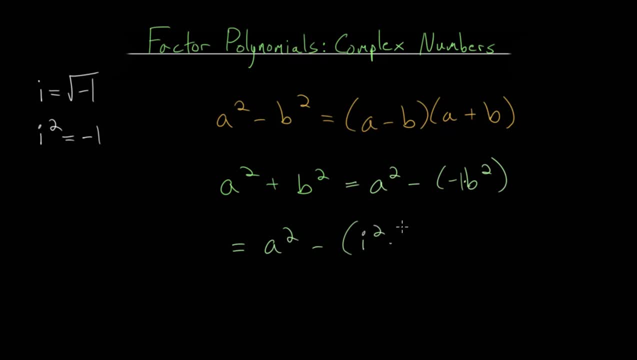 minus a squared, minus a squared. So we have to know all this stuff And now we start concentrating on the final result. OK, so that's going to be a number of lecture sheets right From my requests, and they're both squared. we can rewrite this as a squared minus i times b squared, And you can. 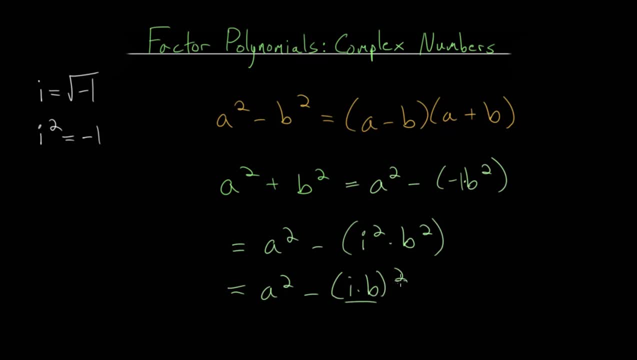 verify that this is true by multiplying ib times ib, multiplying it by itself, and you will get back i squared times b squared. But notice that now we have this difference of squares and we can apply the formula where, in this case, this is like our b from this formula, So we can just plug. 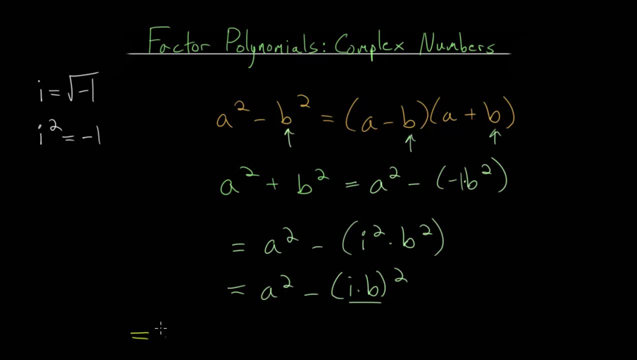 everything in and we will get a minus- this expression without the square- multiplied by a plus- this expression without the square ib- And we can verify this just to make sure that this actually makes sense. So let me just make a little bit of room here. 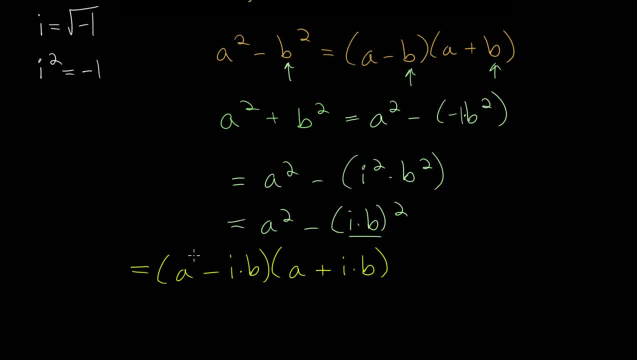 And we'll verify this. We'll verify this by just multiplying it out. So we'll multiply a to both of these terms and this minus ib will multiply both of these terms And we get a times a, which is a squared a times ib. 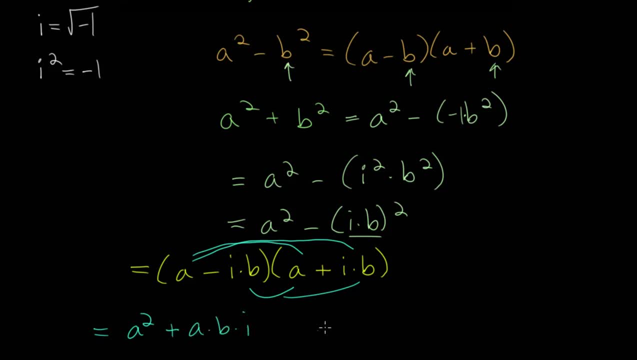 which would be plus ab times i, And we would have minus ib times a, which would be minus a times b times i. And lastly, we have minus ib times, positive ib. So we get i times i, which is i squared, and b times b, which is b squared. 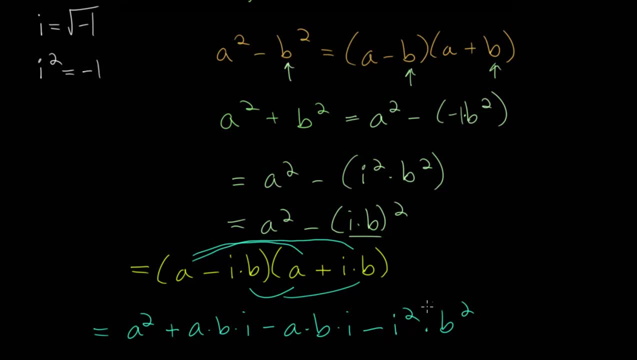 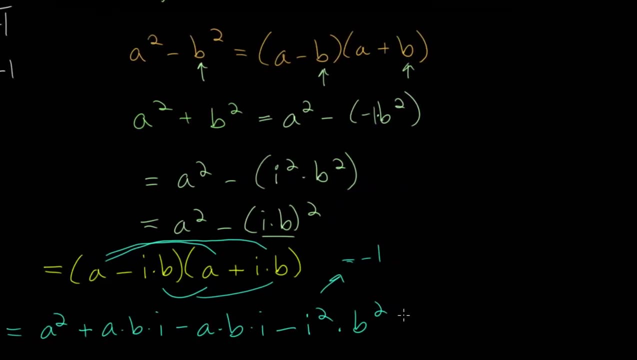 Now we know that i squared is negative one, So we can just substitute that in here- And let me just make a little bit more room over here- And we'll continue working. So notice that the middle terms with i in it, the imaginary terms, these will cancel out. So we just get a squared, a squared.